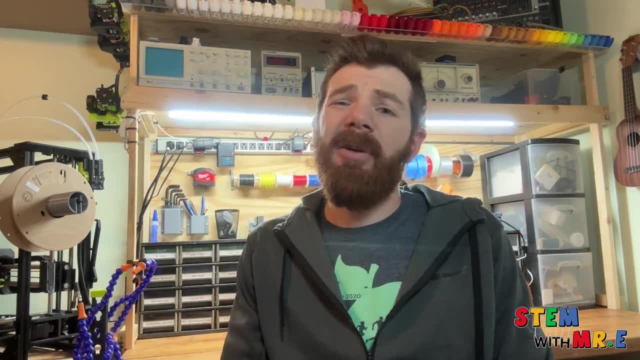 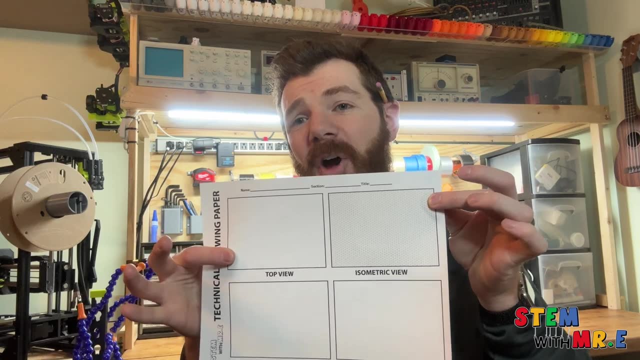 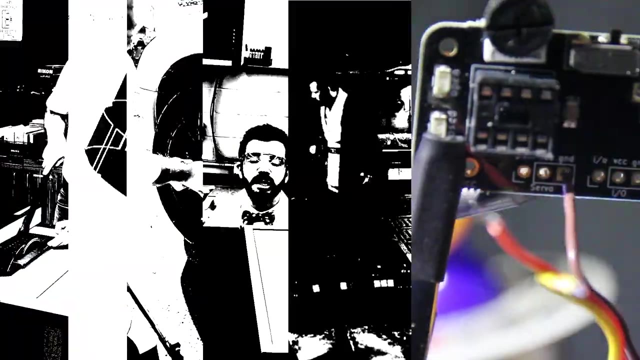 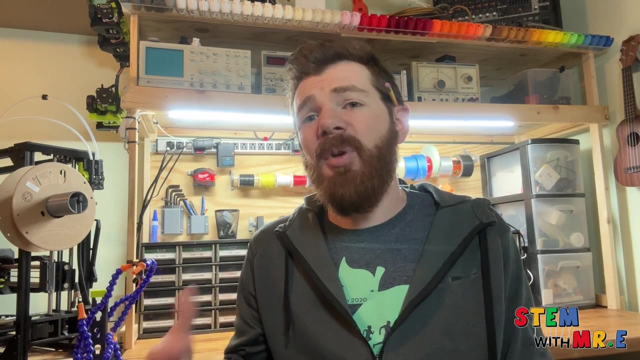 Hey everybody, Mr Urgeis, here and in this video, I want to show you how to communicate your ideas effectively through a universal language for sketching technical drawings. So as we invent and create things and we want to explain those ideas and inventions to our peers, 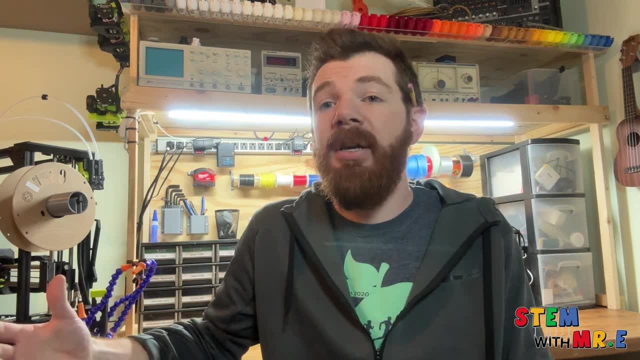 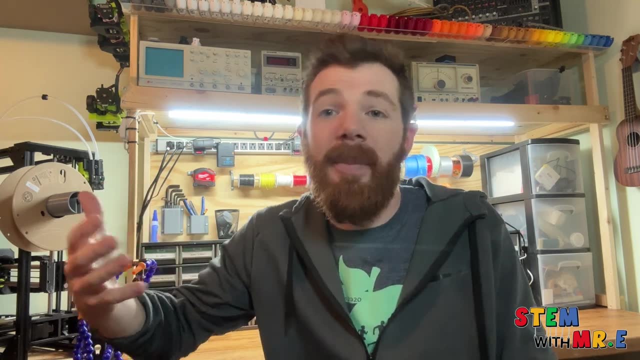 our classmates, our friends, our family, ourself, a machine. we can't rely on our words. If I say I have the coolest invention for a chair ever, you're thinking of a chair, but it might not be the kind of chair I'm thinking of, because the word chair could mean so many different things. 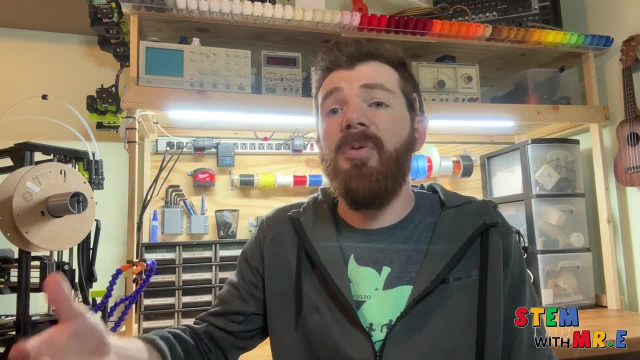 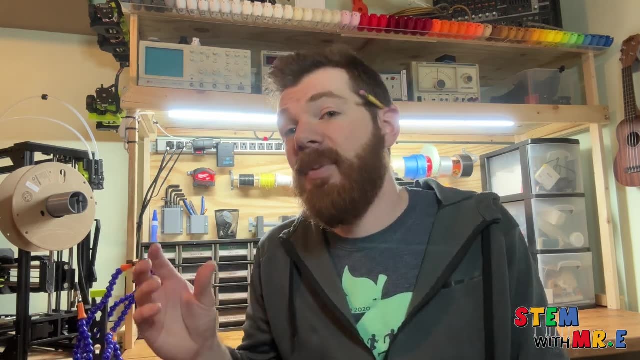 So how do real professional designers share their ideas and communicate what something looks like, something that we might want to build or manufacture, or whatever it might be? They sketch it. Sketching, of course, can be art, but sketching is also one of the earliest forms of 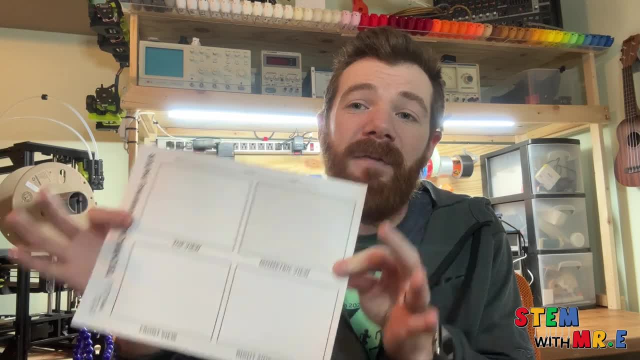 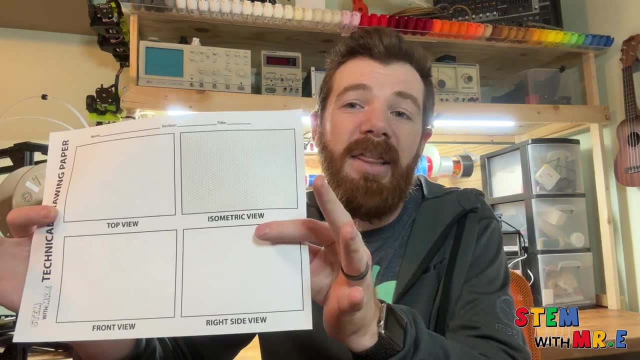 communication And a technical drawing is a universal format for sketching that presents the way that something appears in a variety of layouts. So that way, if you were to look at this- obviously not this, this is blank, but this by the end of the video- you might know or be able. 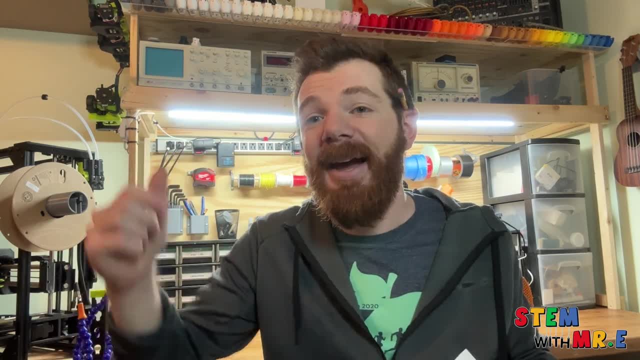 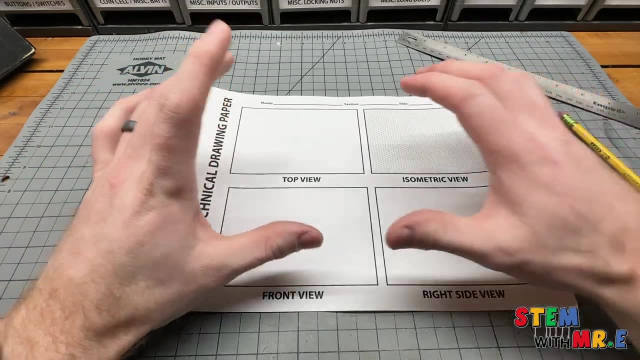 to visualize or even be able to manufacture my idea. So let's dive in and see how to do this Now. as I mentioned, this is a universal language, So, for example, this is a standard blueprint or template that's used in all different types of design, from architectural design to product design. 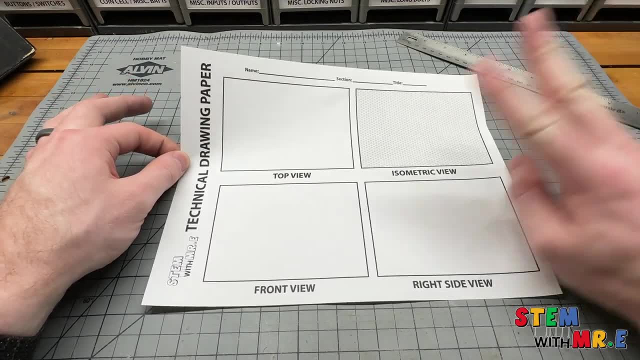 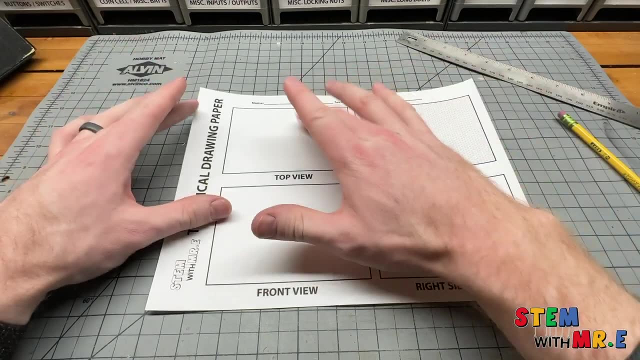 to hardware design and more. There are three major components of a technical drawing: Orthographic sketching, which is where you take an object and you draw in just 2D from different views- typically front view, top view and right side view. And isometric sketching, which is a 30 degree. 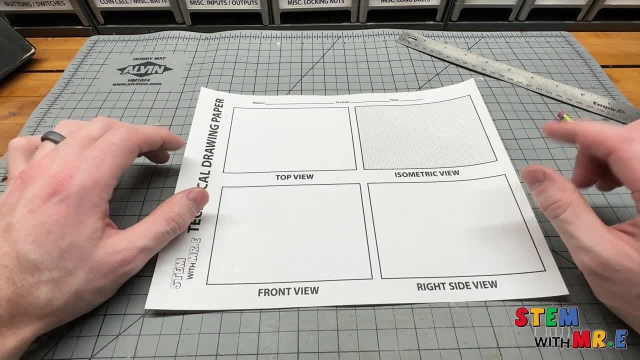 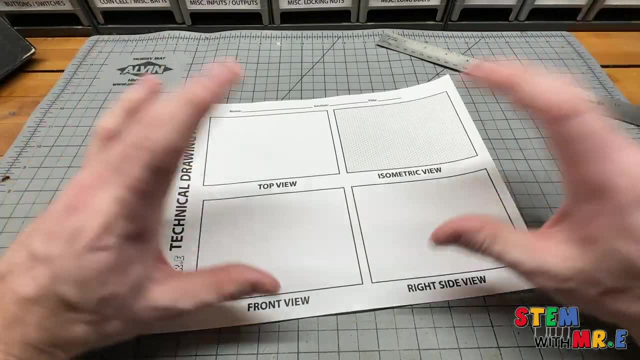 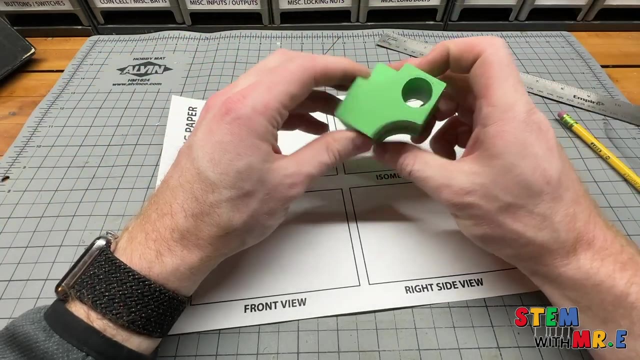 perspective view of what it looks like in 3D and dimensions or measurements. So how big something looks like in 3D? Well, I'm going to hand this technical drawing to you and you would be able to manufacture whatever's on this sheet. Now, instead of drawing something completely random, I'm going 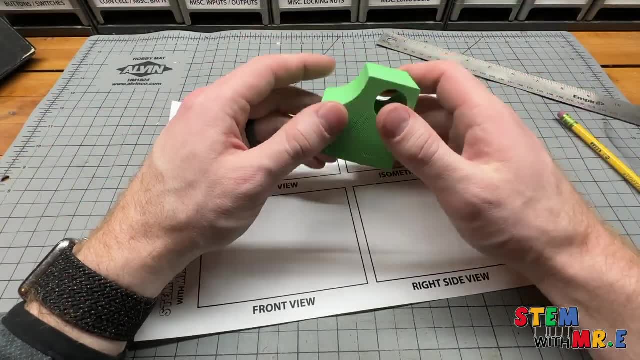 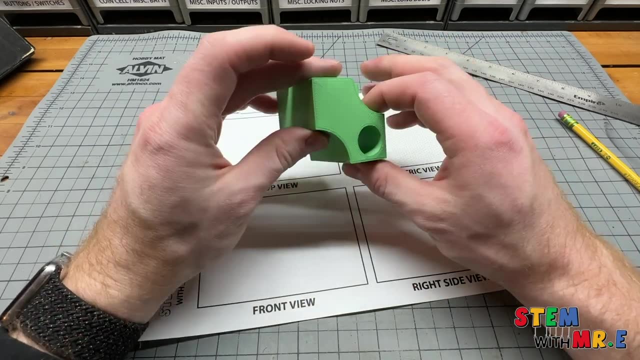 to draw one of my technical drawing cubes. You can grab both this planning sheet and a bunch of 3D printed technical drawing cube files from my website at MrUrgeReichcom. Now the first thing I need to decide is what is the front of my cube, And typically the front of objects are the side. 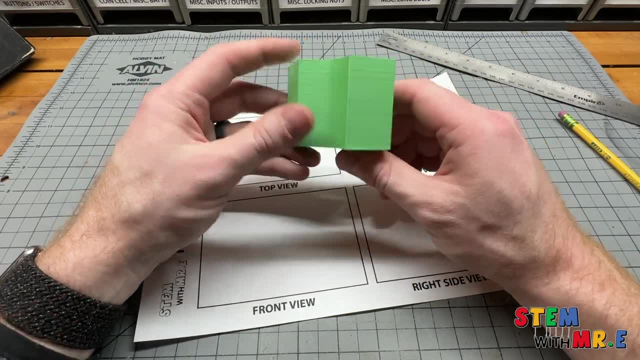 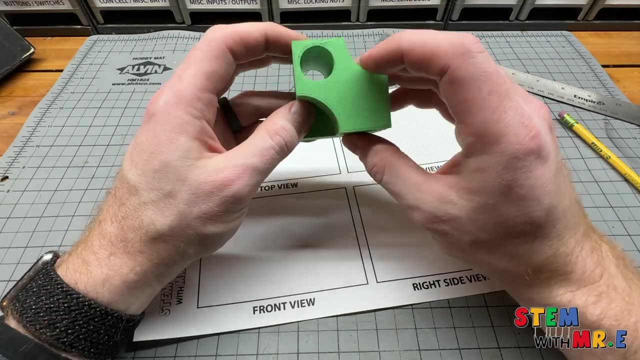 that you interact with or the side that gives you the most information. So, looking at this cube, I have a rectangle with just kind of a curve, a rectangle with just kind of a curve, and right here I have a curve, a hole and another curve. So I'm going to say that this is my front view. Now 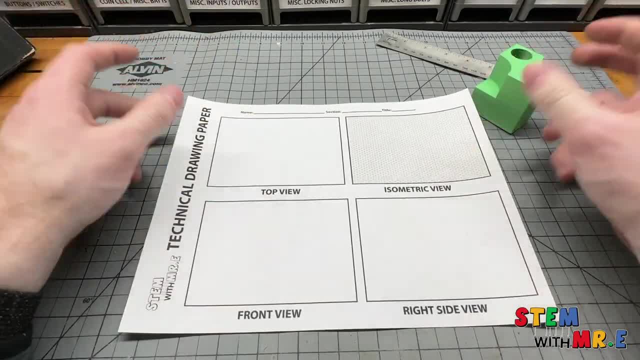 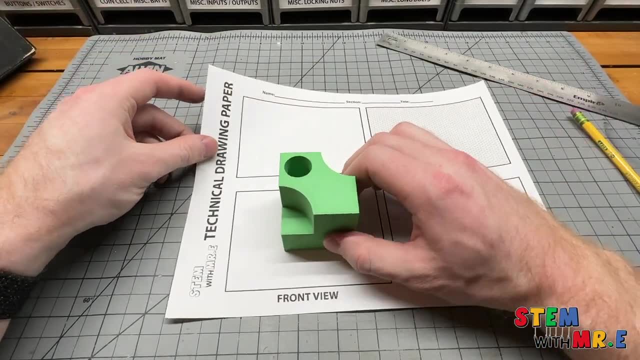 technical drawings can be to scale, or they can be scaled down or scaled up. I could trace over this cube to help draw it. Whatever it might be, the main thing to keep in mind is that you should draw your technical drawing nice and neat. So I'm going to start with my orthographic sketching by 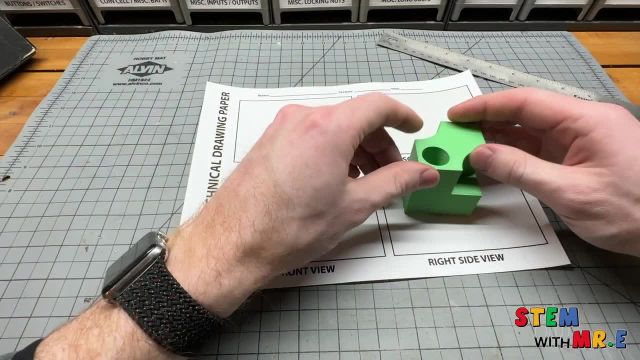 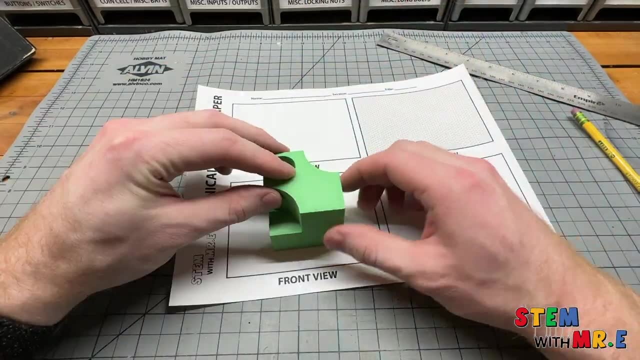 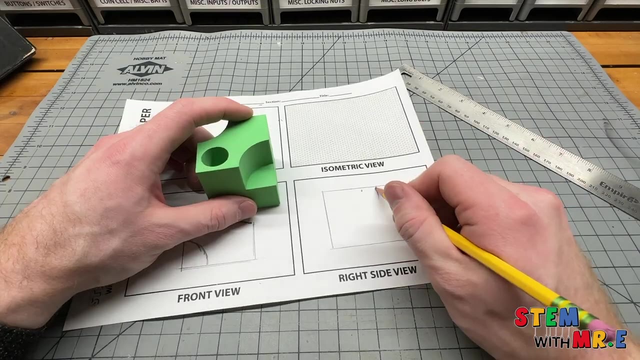 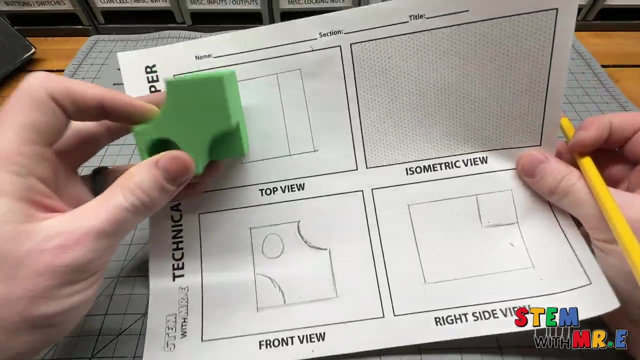 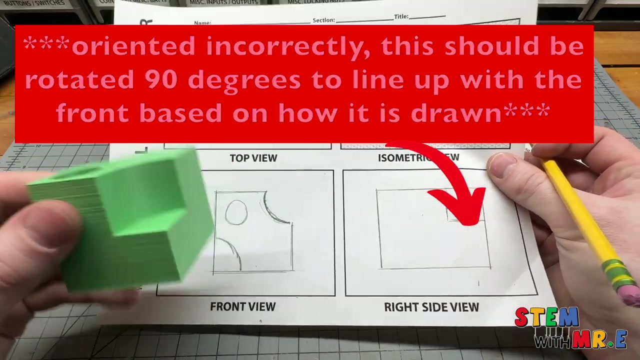 drawing this from the front, the top and the right side view so we can see what this looks like. Okay, so here we go. Here are orthographic sketches of this cube that have been flattened. So I have my front view, I have my top view and I have my right side view. Now, when you're looking at an 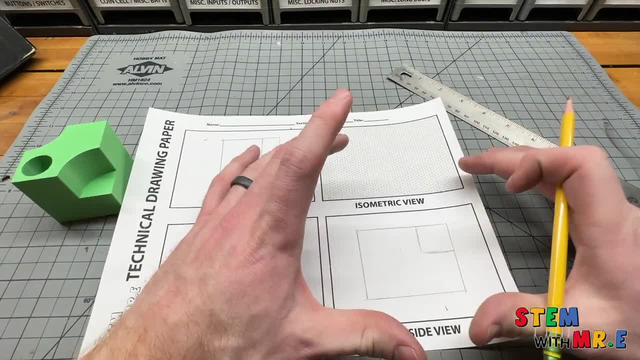 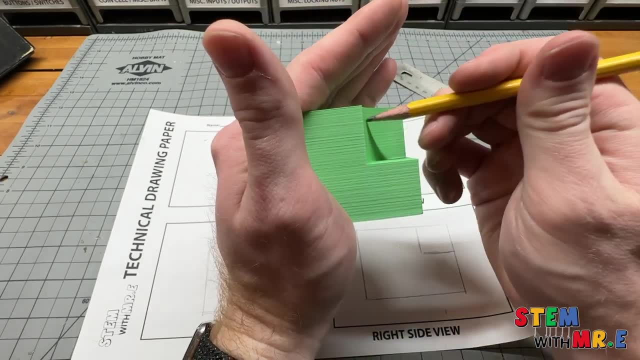 orthographic view or just a single one, you don't get the entire picture. So, for example, from the right side view, when it's perfectly flattened, you can't tell that this is a dished curve. I can see that there's some type of cutout here. I know that this is not connected to this. 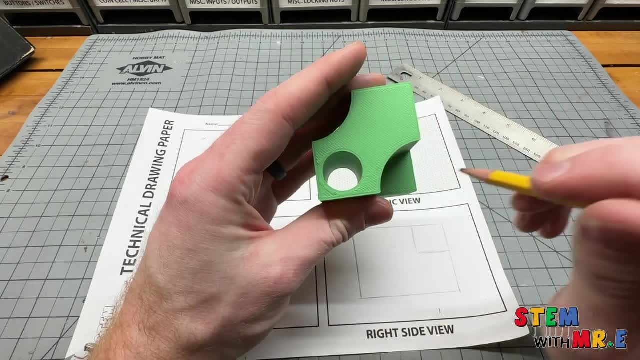 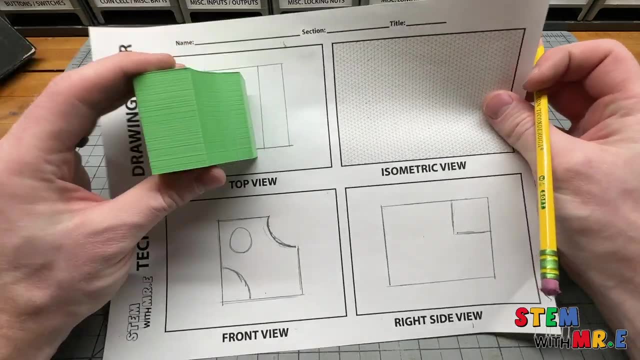 and I've drawn that, but I don't get to see that it's actually a curve until I look at it from the front view, From the top view, it's the same story. When I look at this from the top, I can see that this is not connected. so I can see that there's some type of depth. 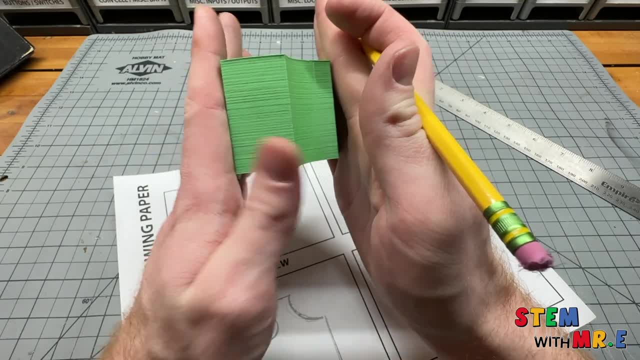 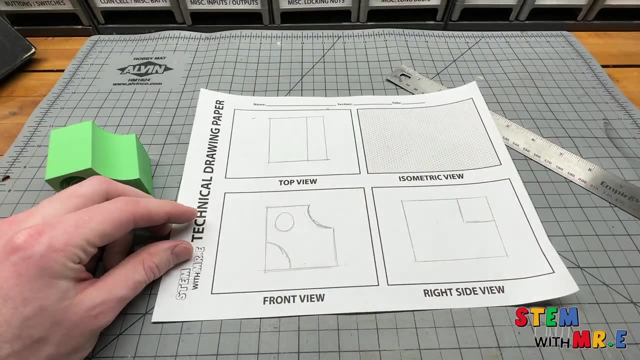 Because I can't see the depth of this dip when looking at it in just 2D, it's just simply drawn as a single square. Now, two important things to keep in mind is that you should always line up your views. So I did what's called projection lines, where this and this is lined up across my views. 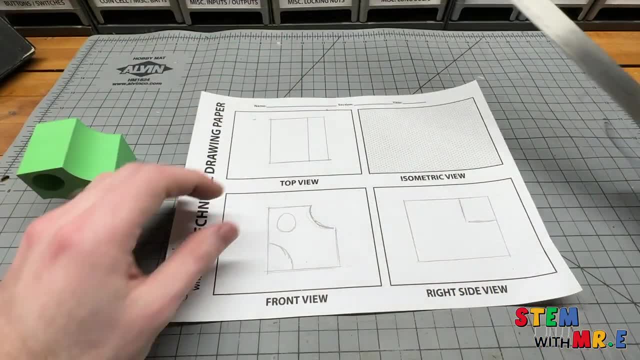 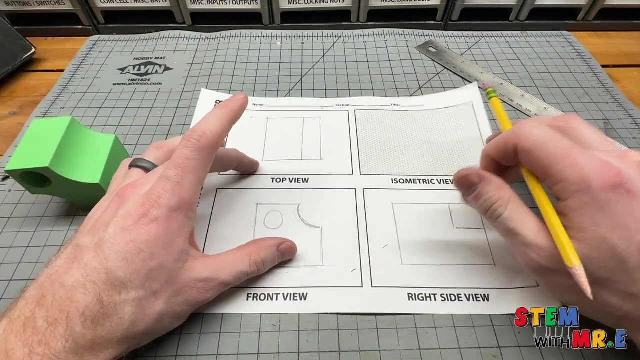 to make sure that this is perfectly in line here. The other thing you should do is always draw in pencil, so that way, when you make a mistake, you can easily erase it. So now that I have my orthographic drawings, I'm going to go ahead and add my dimensions to this by measuring the 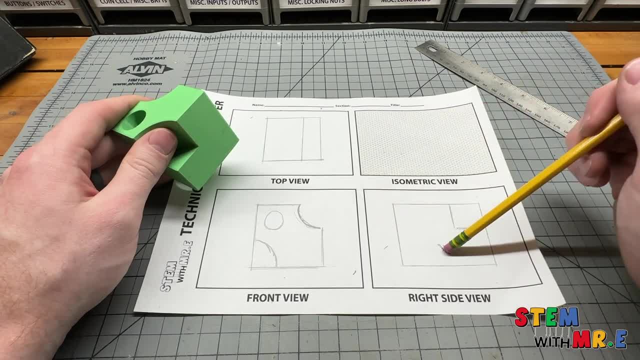 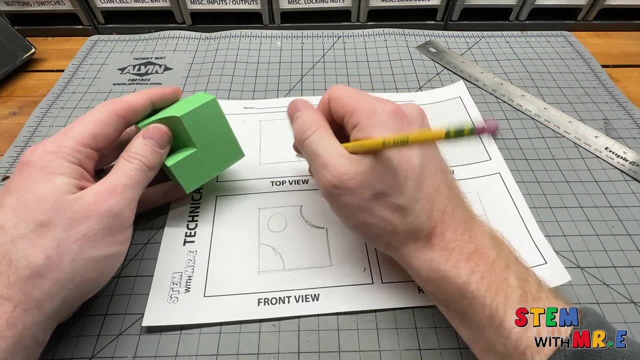 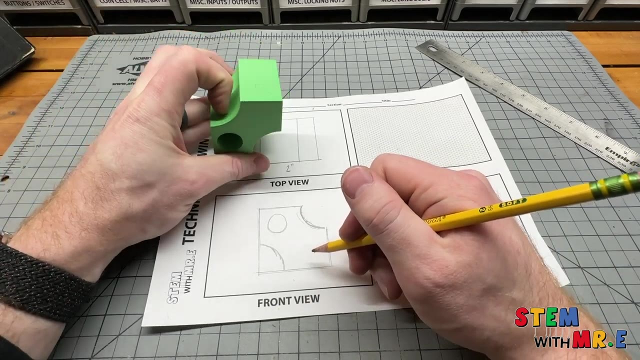 different features, And the cool thing about this is that this is the same shape from different views, So I can share measurements. For example, I know that the width here is two inches. I don't need to put the width here, because if it's this wide from the top view, 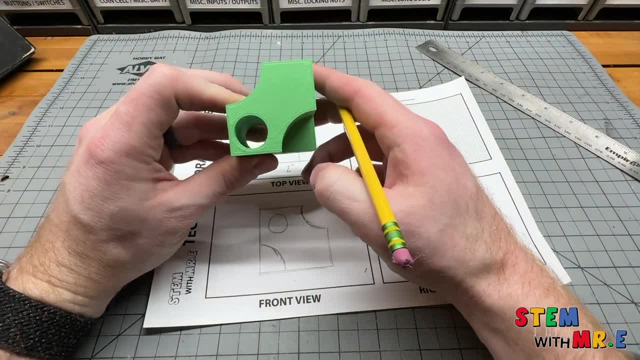 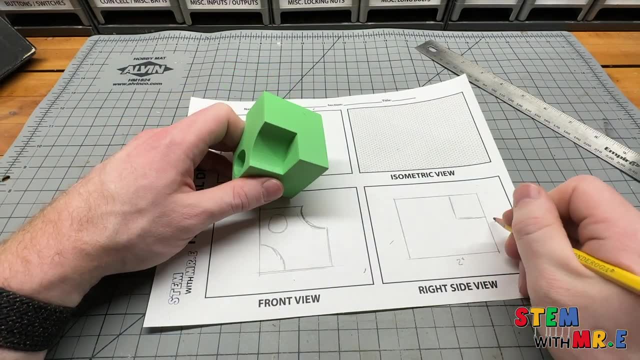 like this: then it'll be the same width from the front view But the depth might be slightly different. So when I draw my right side view I need to label this to be two, But I can share the height. So if I put two here on the height here it's not going to grow between different. 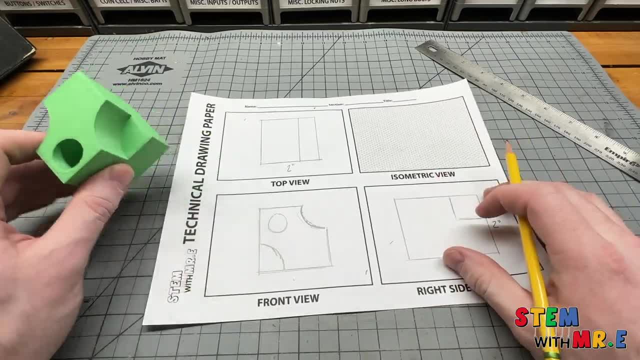 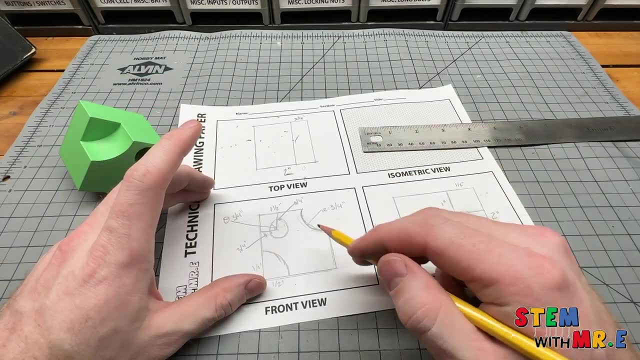 views So I can share my measurements as I work my way around. So I have my measurements and it doesn't look like a lot, but again, that's because I'm able to share measurements across my different views. Now, when you have a hole or something like this: 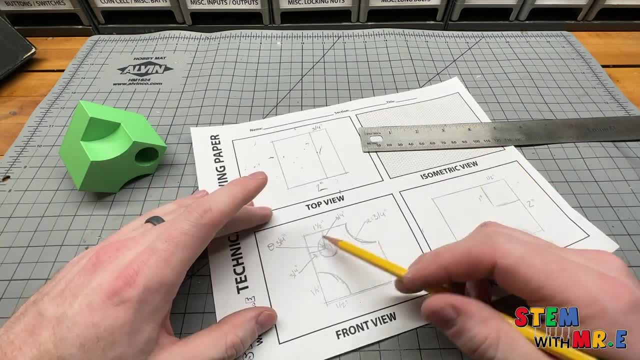 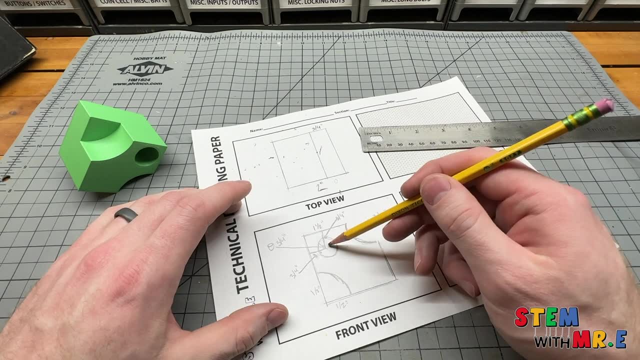 you've most likely needed three measurements. What is the diameter or the radius of the hole? And I start to run out of space, so I use arrows to label where things were And also where is the hole located. So on a 2D plane of all shapes in space, any object or cut has two positions. 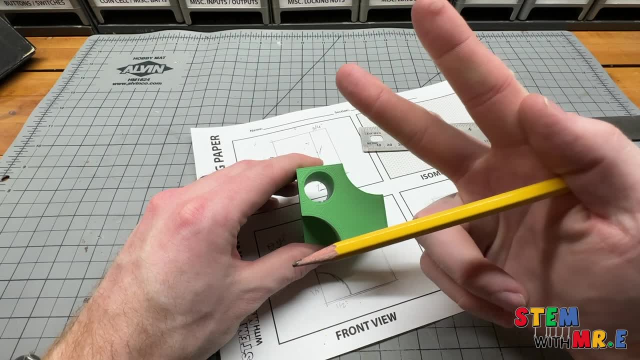 When I do 24,, 7ne brings into my model the same as the red representation was in the second plane. So that's in focus. But when I draw the AA objective I get just 5.. If I go from there, that's the same difference. 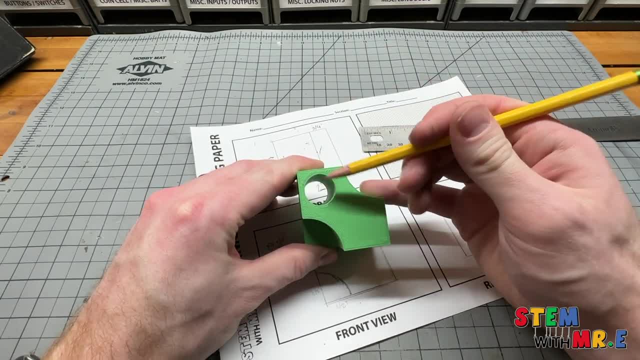 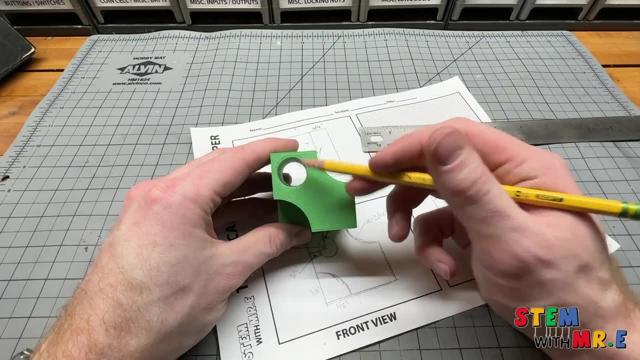 an X position like this, which would be its horizontal position and a Y position. So, measuring horizontally from an edge, I put that measurement. Measuring vertically from an edge, I put that measurement. So if I gave you a block of wood and asked you to manufacture this part, you would know. 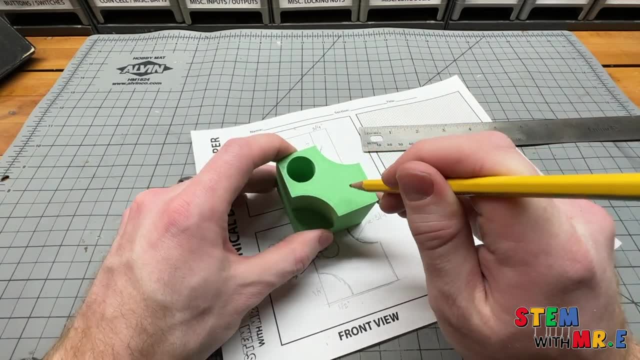 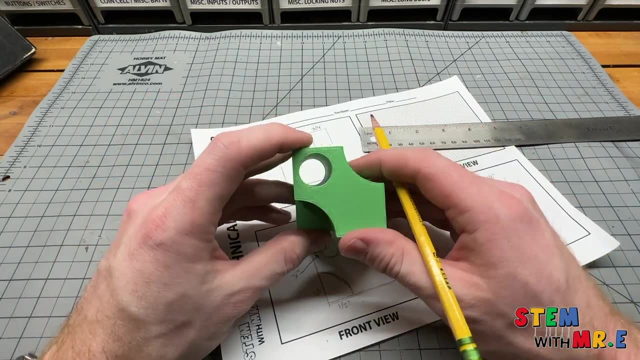 the curve size here that you would need, but you'd also know where to plot the center point to then drill this hole. So it's really important to have the position of the hole as well as the size. The other question is: does the hole go all the way through? Now, obviously, looking at the shape, 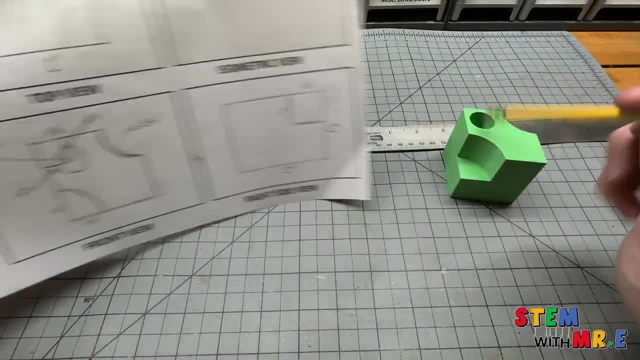 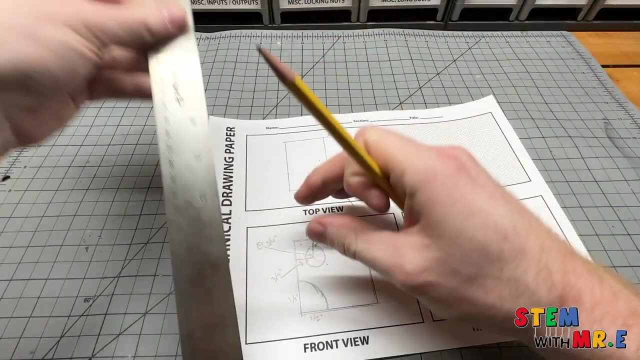 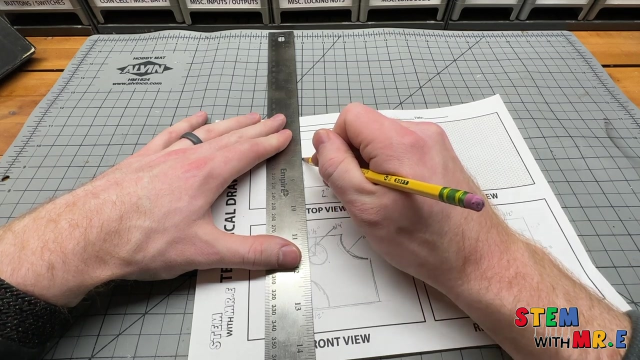 we can see that it does, but if you're looking at this just in 2D, it's really unclear to see if that goes all the way through. One thing that we can use are hidden lines, So hidden lines will plot the path of this hole on other views. So the hole would be cutting through the shape up here. 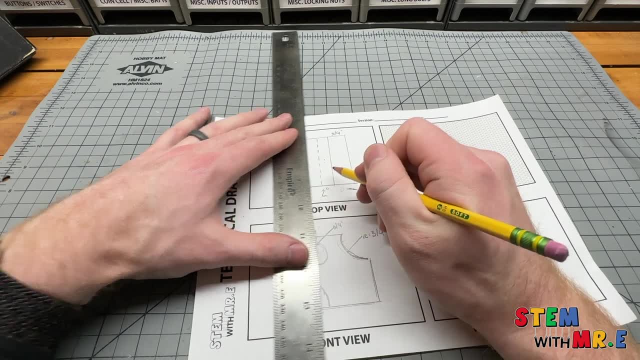 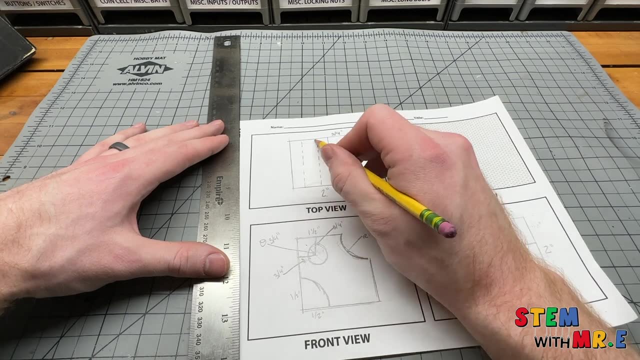 and I'm drawing the path of the hole as if it was a cylinder, using dotted lines. So the reason that there's two dotted lines is: imagine- and you don't want to do this, but imagine that there's two dotted lines and you don't need to draw this- that this is the opening and this is the exit. 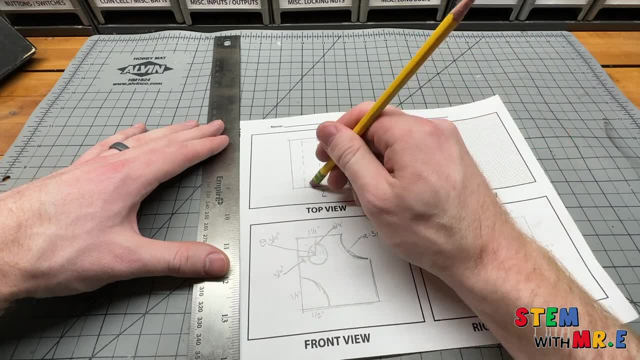 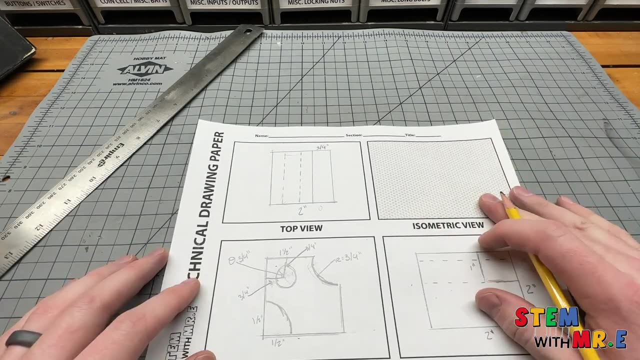 and then this is the boundary of the cylinder that's created with the actual hole, And I'm going to do the same on my other view. Now, the isometric view can be a little tricky. Some people find it easier to draw because this is 3D and your eye sees in 3D, so you can draw it like you. 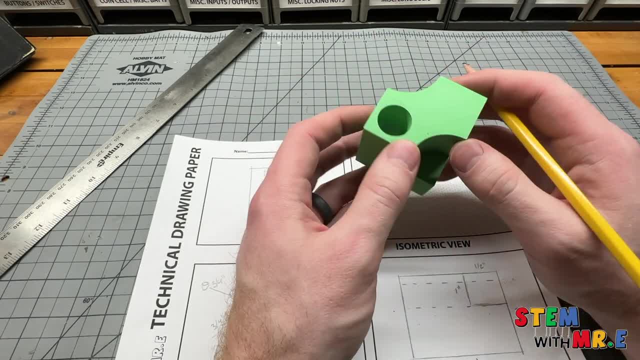 see it, And some people find it to be more challenging to draw because it is a little bit more on the artistic side. But again, the goal is not to create a hyper-realistic sketch of this, but to show you what the actual hole looks like. So I'm going to draw this in 3D and I'm going to 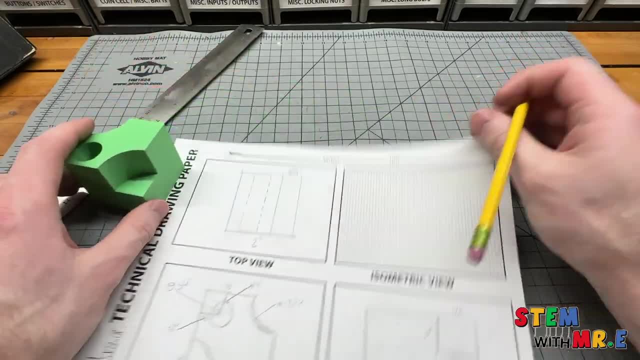 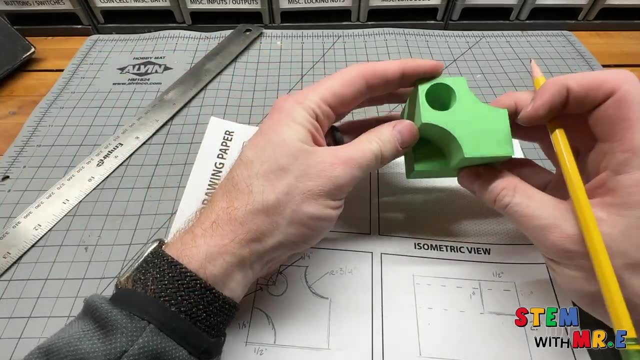 show you what this would look like, as if it was sitting here on the table. So I'm using an isometric drawing grid which alternates between 30 and 90 degree angles, which allows us to create this three-dimensional perspective view. So the first thing we do is I'm going to hold this at 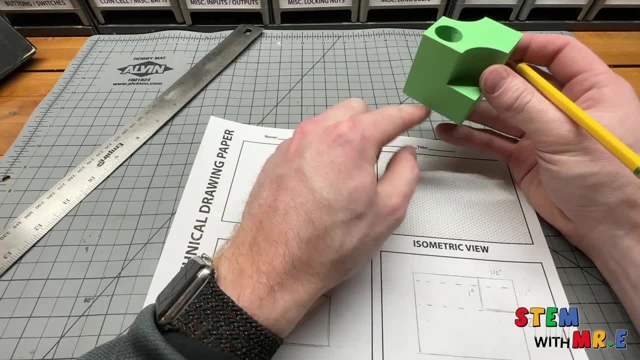 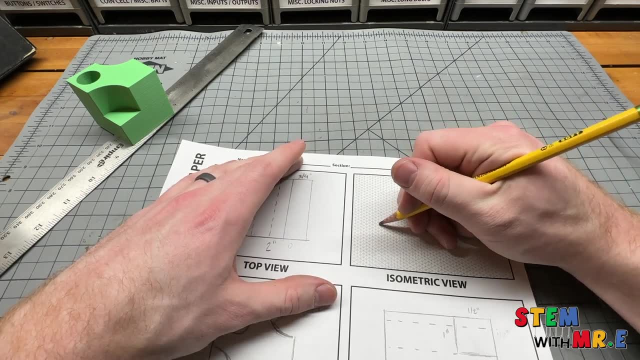 roughly a 30 degree angle and I'm going to pick an angled line. so this bottom edge to start with. So I'm going to start by drawing this angle of the shape right here. So that is a sloppy line. Let me try again. 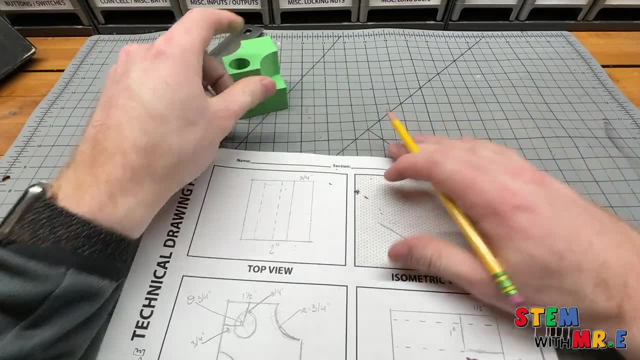 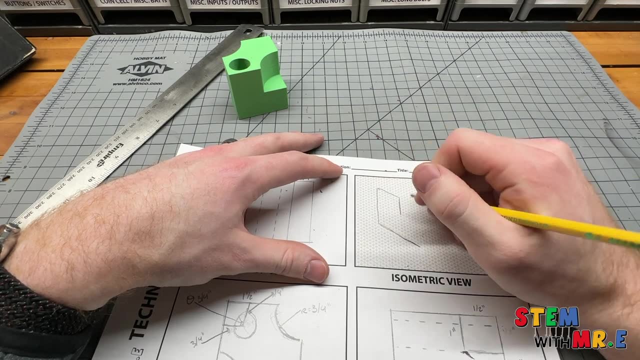 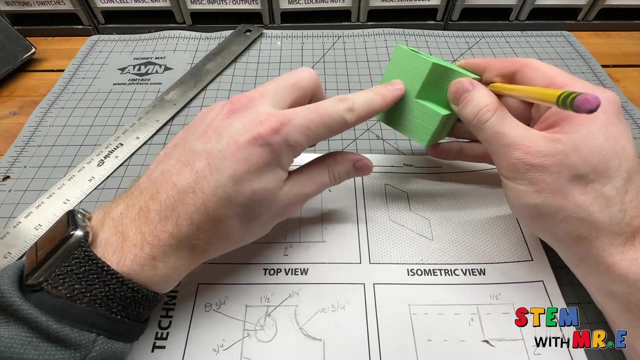 Slightly better. So this is this edge. So from there I can see that it goes straight up, and then it comes over for a little bit and then it comes straight down. And I'm changing my perspectives as I work line by line, drawing my shape. I've now drawn this entire side From 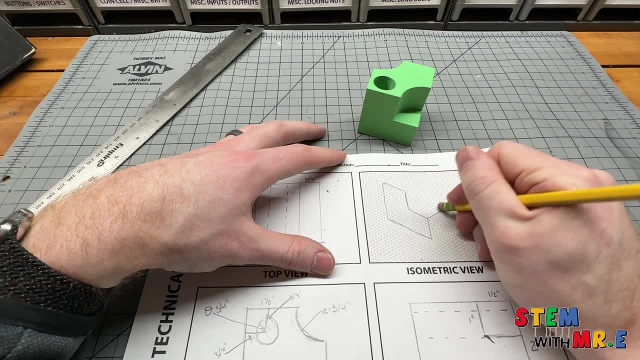 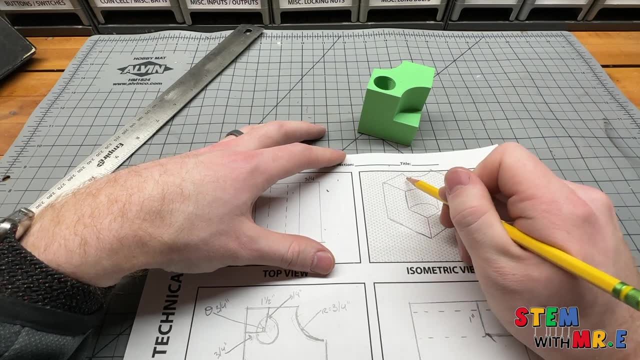 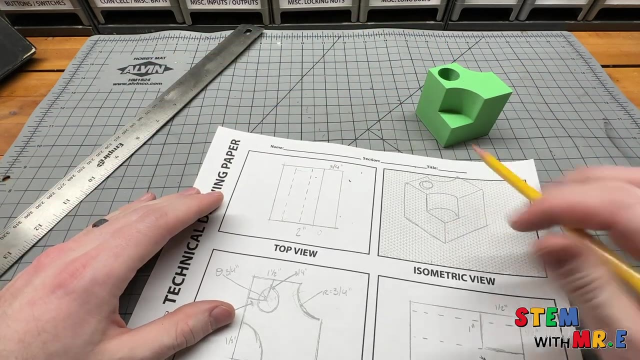 there I have to come in- maybe not that far- and up connecting my lines and erasing when I make a mistake. Really cut it close on this drawing here. But that is my cube Now. you don't ever want to put measurements on your isometric. because this: